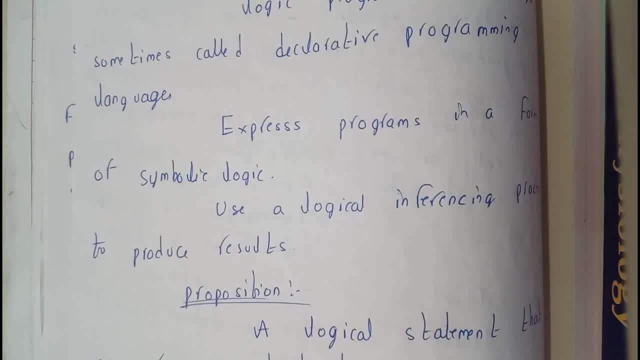 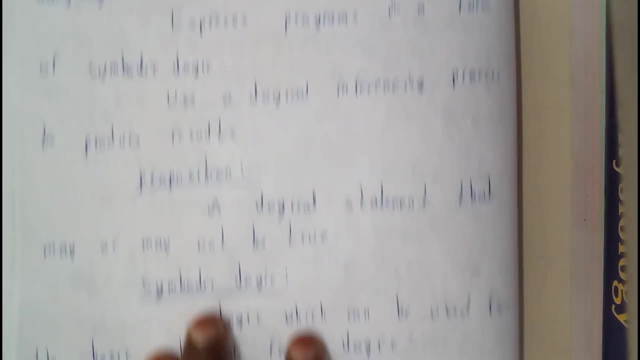 already discussed in discrete mathematics itself, guys. So in our previous lecture series in semester 3 we have discussed that, So now let us go through this topic. So in this topic we are having proposition, A logic statement that may or may not be true. 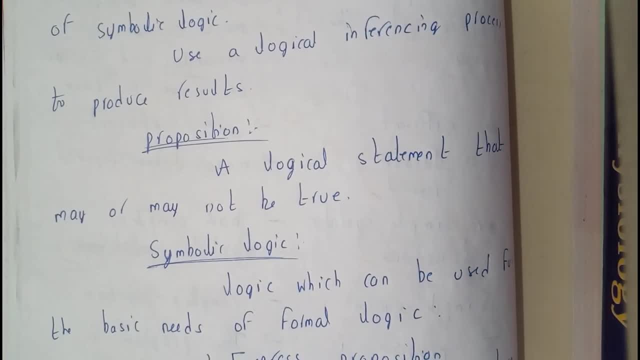 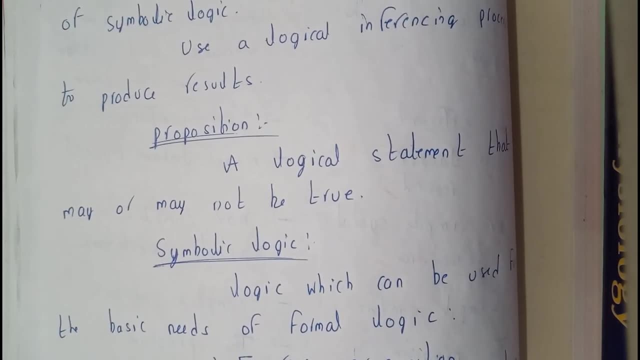 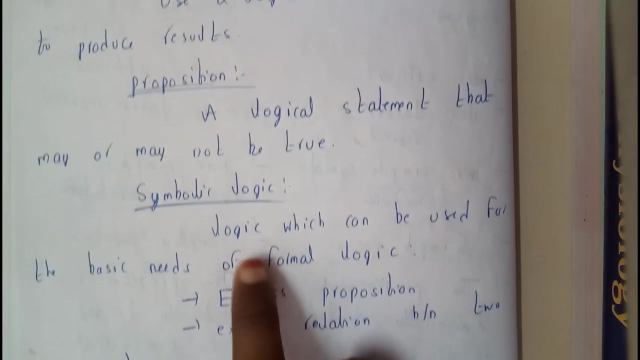 Okay, let us assume P and Q is equals to R. Okay, if you want, in statements Today it may rain, It may or may not. So it is true or it may not be true. So this is called as a proposition. Fine, Okay, So symbolic notation Logic which can be used to used for the basic. 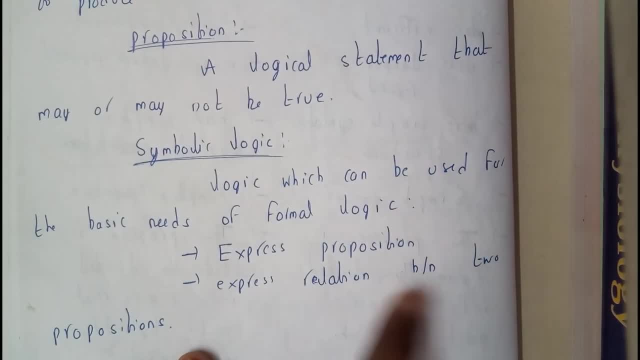 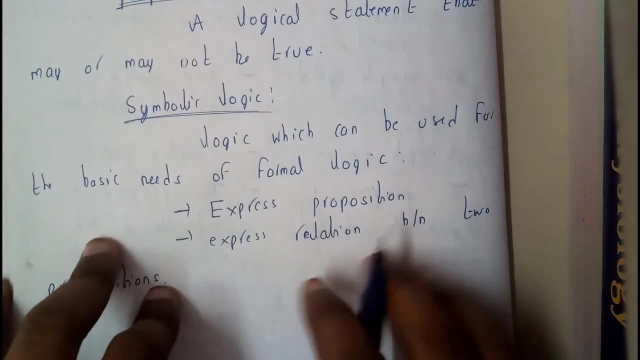 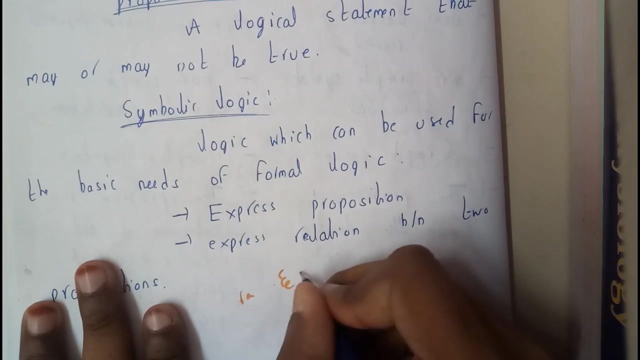 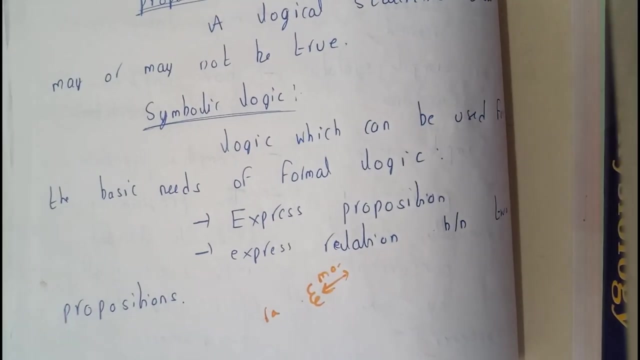 needs of formal logic. That is, expressing a proposition, expressing a relation between two propositions. So fine, So now let us assume two statements: If it rains today, if it rains today, then only I will go to movie. Okay, So only if it rains today I will go to movie. So this relation. 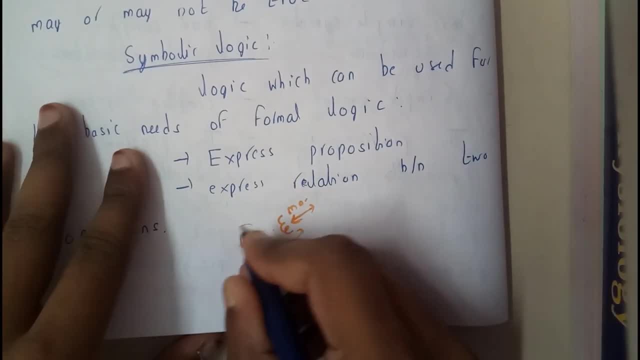 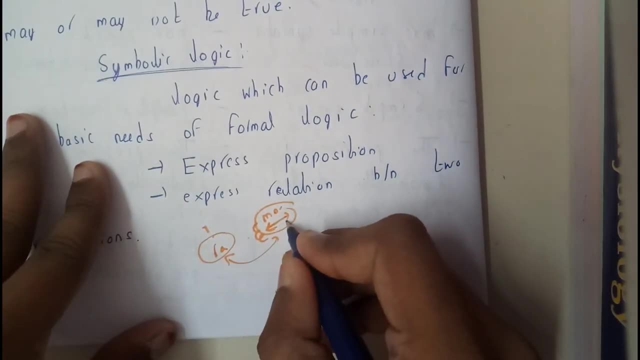 will be something like an and operation. If it is raining, only then I will go to a movie. So the final result is: If it is one, then if it is raining, only then I will go to a movie. So that is in relation. 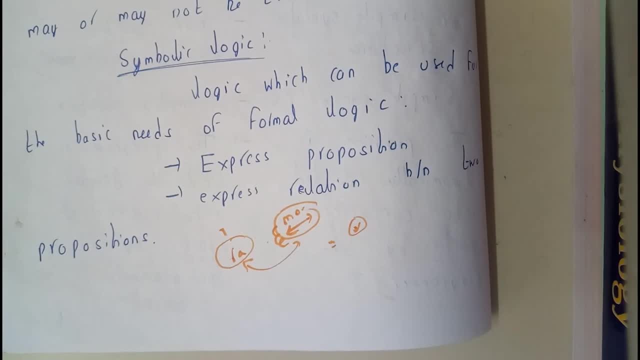 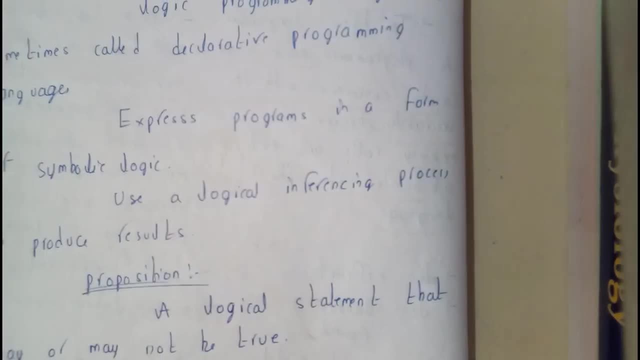 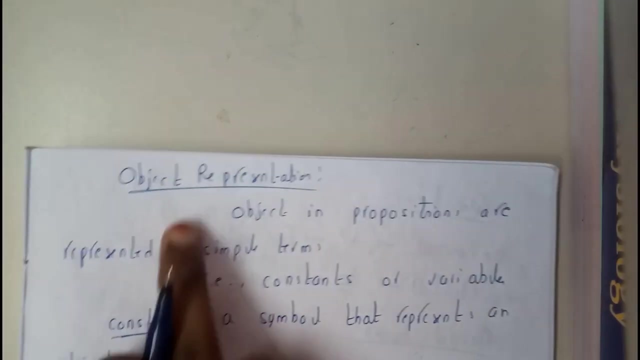 like this, guys. So now I hope everyone got a small idea on this. So just give me a second, guys. I will be back in a second. Okay, so these kind of representation is nothing but symbolic logic, guys. So representing them in symbols, So we are having object representation. 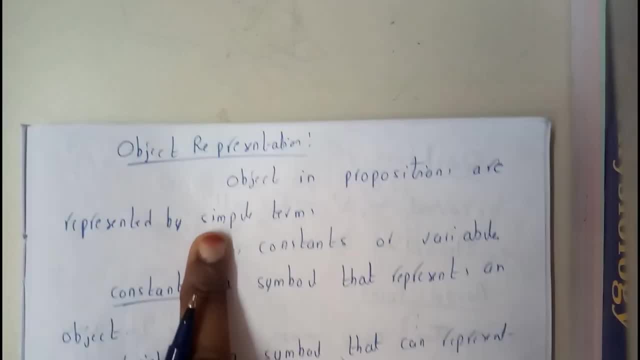 also. So object is a proposition or representation of something. Okay, So this kind of representation is nothing but symbolic logic, guys. So representing them in symbols. So we are having object representation or representation of something. Okay, So this kind of representation is nothing but. symbolic logic, guys. So this kind of representation is nothing but symbolic logic, guys. So representing them in symbols, So this kind of representation is nothing but symbolic logic. Okay, So this kind of representation is another sort of representation. excuse me, but there is another sort of representation. here instead of symbol, and that's not symbolic logic, guys. So this kind of representation is an object, a value of object or a variable sharing a component, a function or a variable that is represented by simple terms. So it can mean: now, Xiaomi, higher than that symbol. 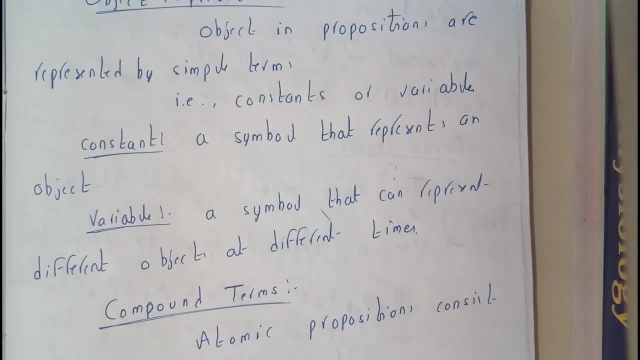 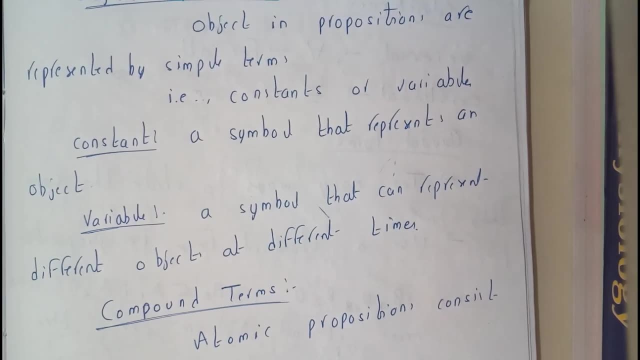 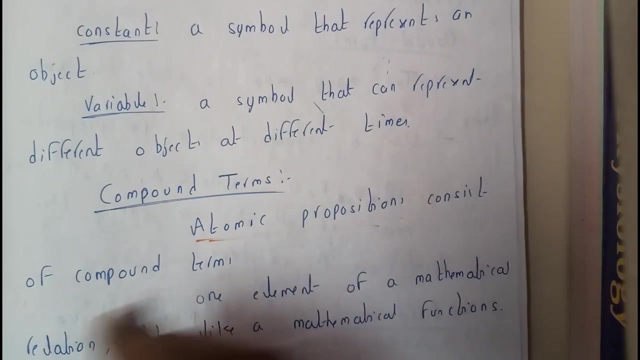 here The original wise, you can inherent to rigid attributes. that Doctor is always taught on here. however, this is something very different. now you have to learn it in theclock of the super surface object. But when the temperature goes down, what over it does? here whatât? 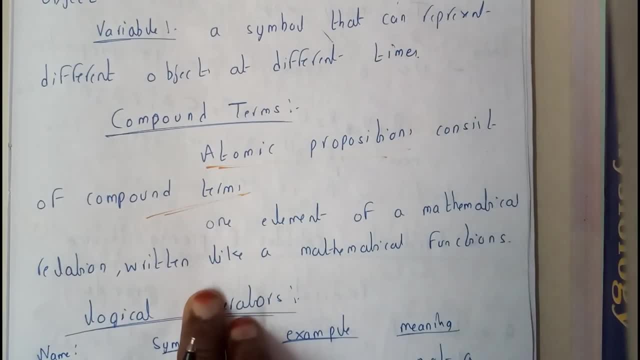 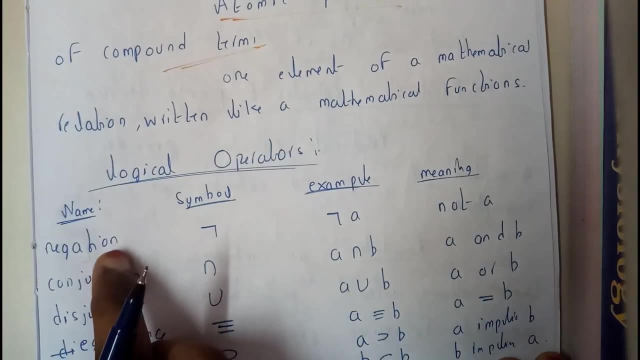 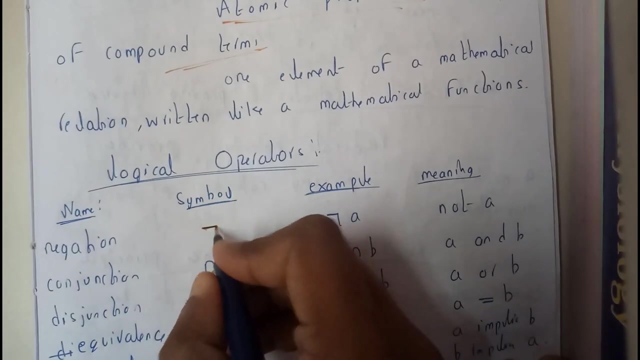 components, so one element of mathematical relation, return like a mathematical function. so logic, logical operation operators are nothing, but we are having the symbols here, guys. so negation, seven, sorry, negation will be like this: guys, this is not seven, but it appears to be seven like, but it is seven, only guys. basically fine. 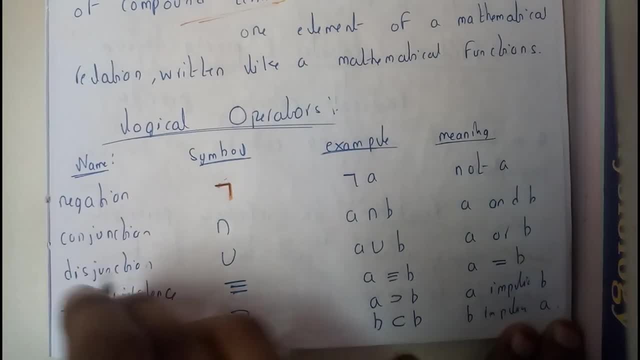 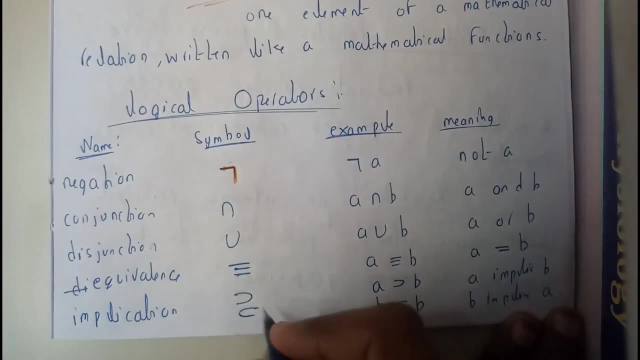 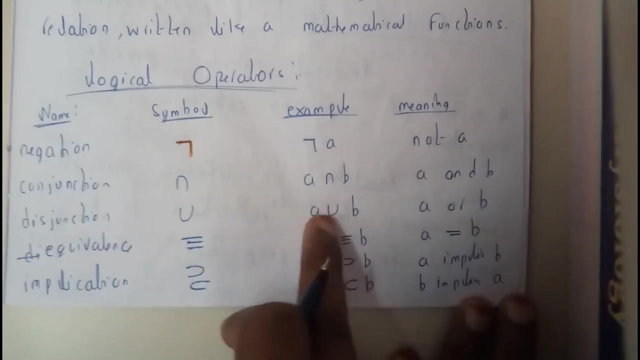 we will be using to denote that with seven only. okay, fine, you can even assume that as seven. so conjugation will be reverse, u disjunction will be, u equivalent will be three, three equal to implication will be one, two, like that. so we so with an example- this is here, guys, not a a and b a. 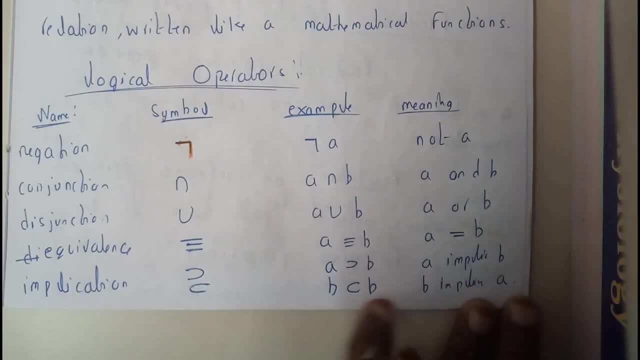 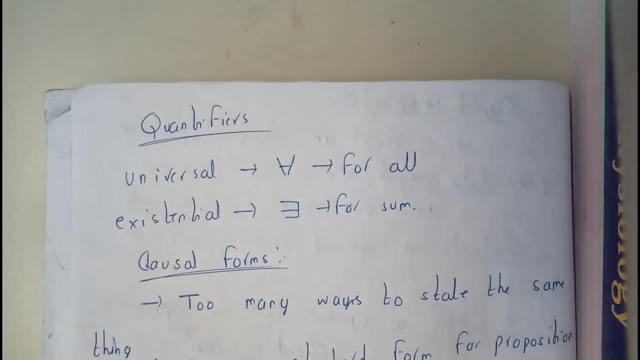 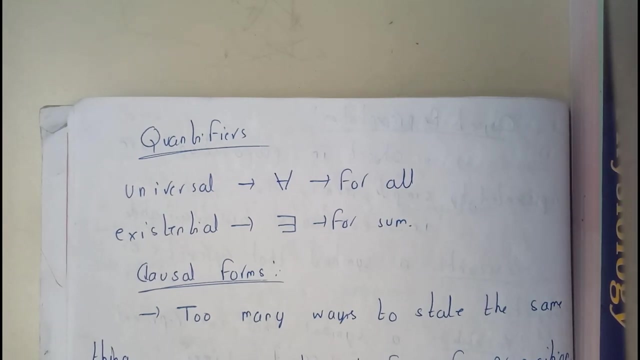 or b, a equal to b, a implies b, b implies a. so this is the in terms of words guys. so now let us go to quantifiers. so these all things we have covered already already in discrete mathematics, guys. so that is nothing but dm. so we have already covered these all things in semester three. so now, 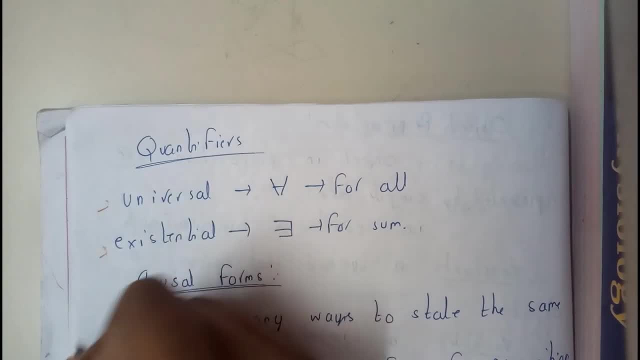 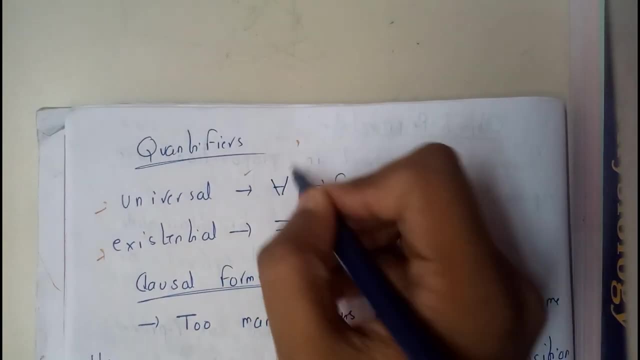 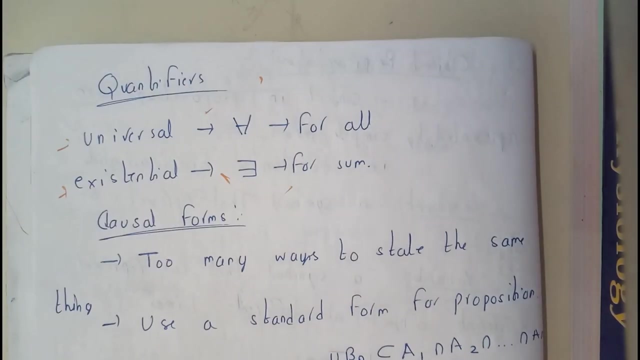 let us go through quantifiers. we are having two quantifiers: universal and extensional. so universal are nothing but for all. so this situation will be for all and this extensions will be only for few. so now i hope everyone got a small idea. and there is one more form, guys, which is one of the 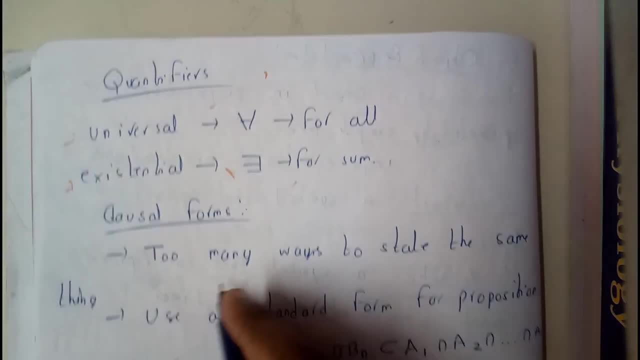 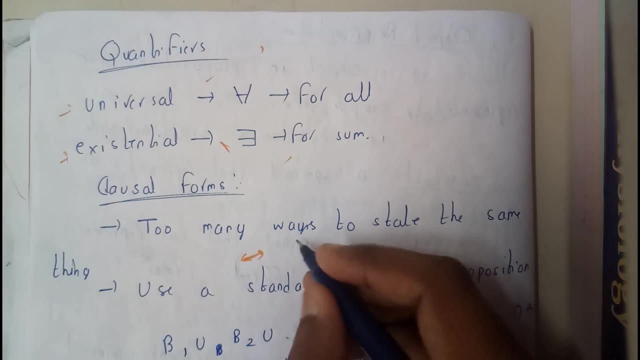 important thing, that is clausal form. that is too many ways to say a state the same thing. so if you want to write a statement or if you want to get the result as nine, and you can do five plus four, you can do four plus five, you can do three plus six. like that there are. 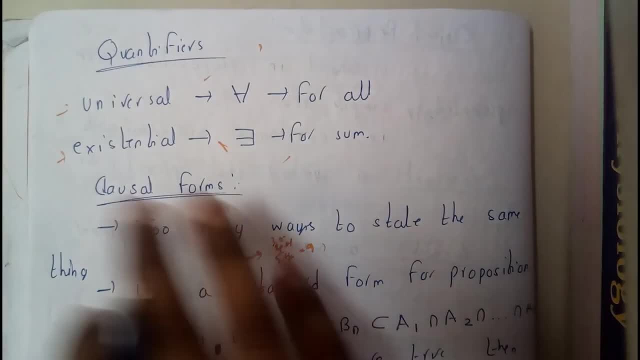 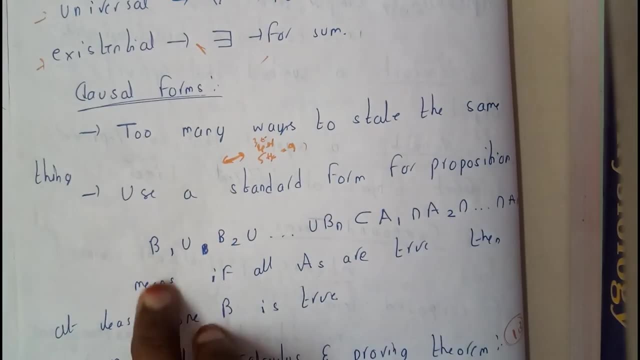 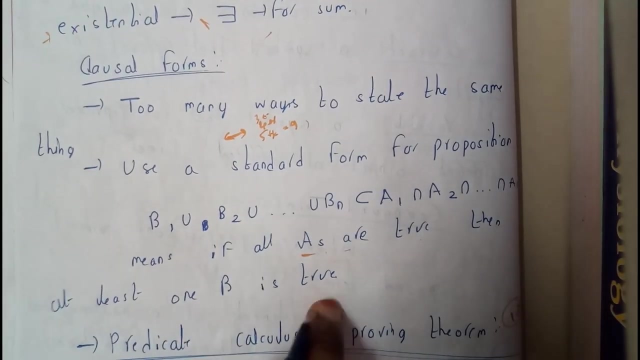 many forms right. so like that also in this, in this propositional formats, also in logical statements also, we are having many forms. so usage of standard form of preposition- this is the format of that. guys means if a s is true, then at least one b is true.